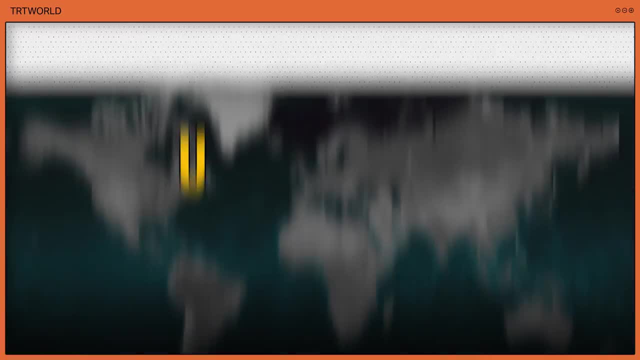 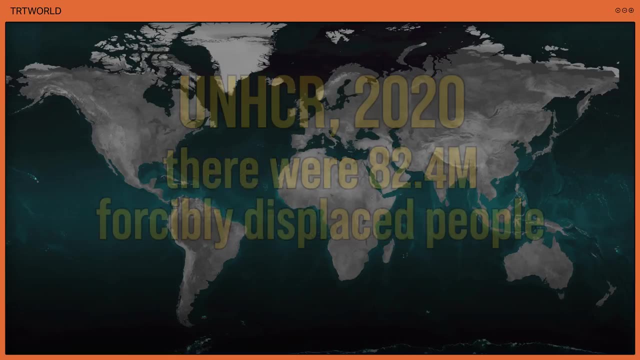 if they arrived- quote- directly from their own country. According to the UNHCR, at the end of 2020, there were 82.4 million forcibly displaced people around the world. Millions of these people should be covered by the Convention, But the ever-increasing number of asylum seekers to 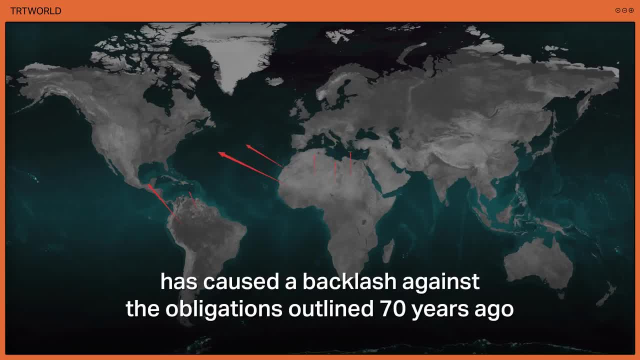 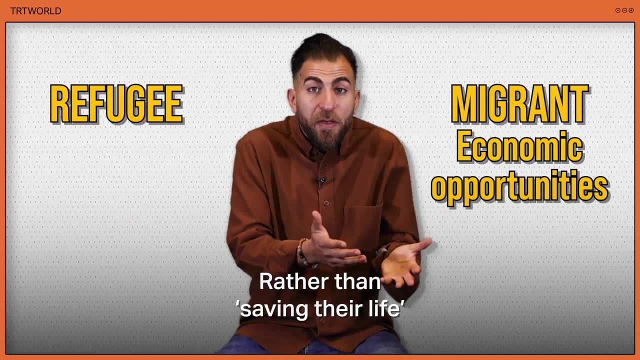 Europe and America has caused a backlash against the obligations outlined 70 years ago. Now, a migrant is someone whose motivation is to improve their economic opportunities rather than saving their life. But the lines are murky, Very murky, In the sense that people who are forced to leave their homes. 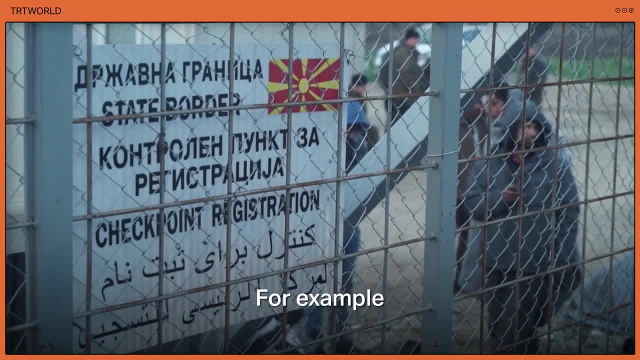 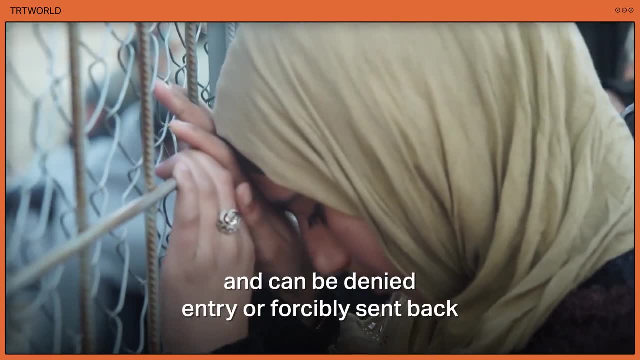 may also aspire for a better quality life. For example, think of a war-torn Syrian who left to Turkey and then once again to Europe through Greece. They have travelled through a third country and can be denied entry or forcibly sent back, as we have seen time and time again. 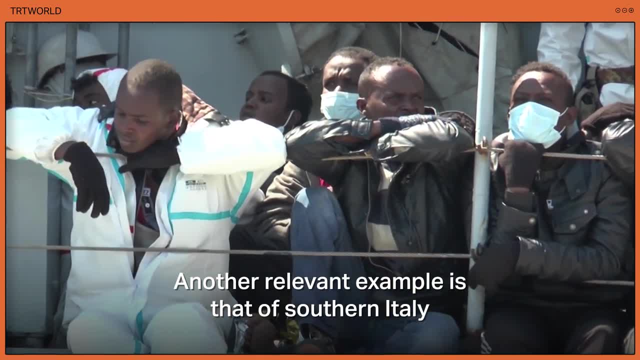 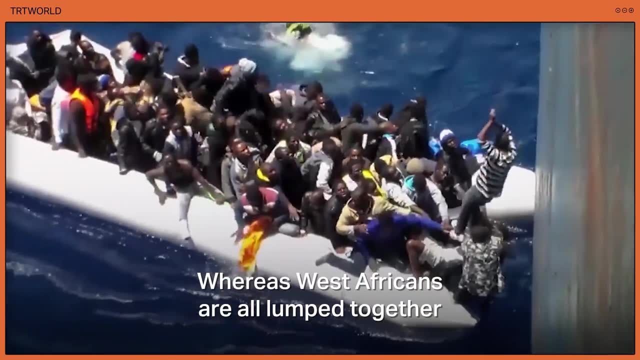 despite him or her being a refugee. Another relevant example is that of Southern Italy. Authorities and the media designate Syrians and Eritreans as bona fide asylum seekers, Whereas West Africans are also forced to leave their homes despite the fact that they have been. 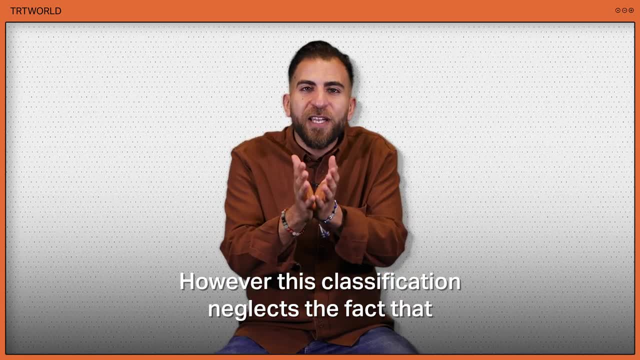 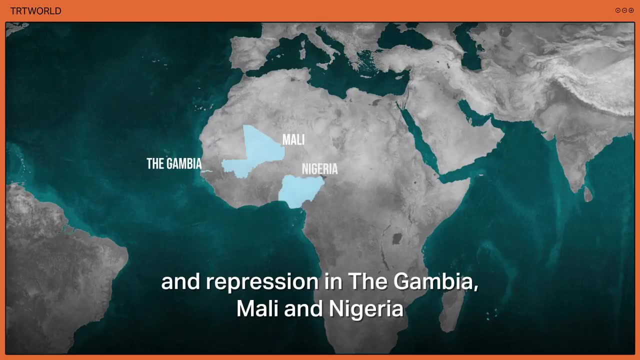 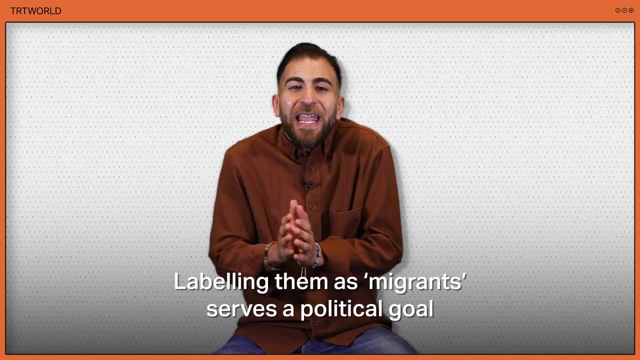 all lumped together as economic migrants. However, this classification neglects the fact that many of these West Africans have experienced violence and repression in countries such as The Gambia, Mali and Nigeria. They have also likely faced arbitrary detention and violence in countries like Libya, forcing them to flee again. Labelling them as migrants serves as a 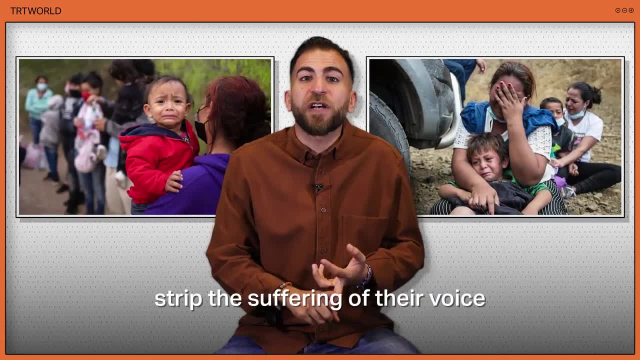 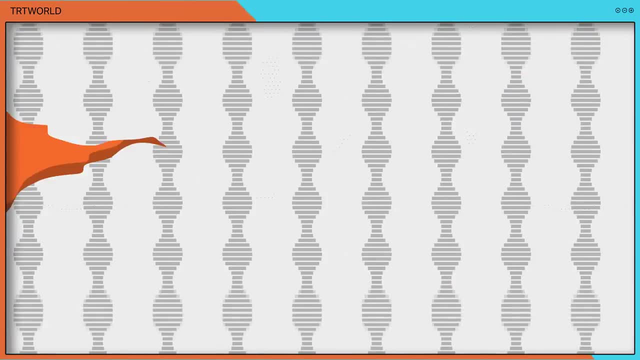 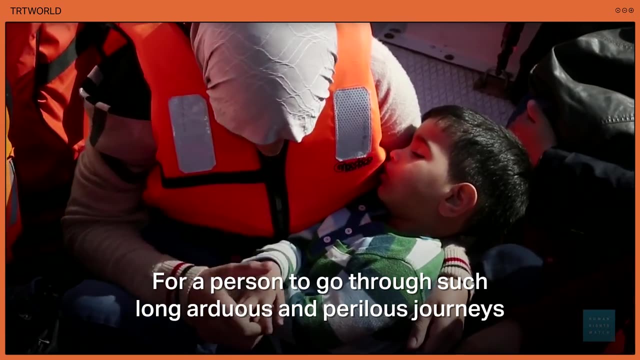 political goal, To detach value from their life, strip the suffering of their voice, excuse their death or deportation and, lastly, to bypass the duties of the Refugee Convention. More than facts, statistics and semantics, we must perceive the human factor For a person to go through such long, arduous and perilous journeys, risking their lives. 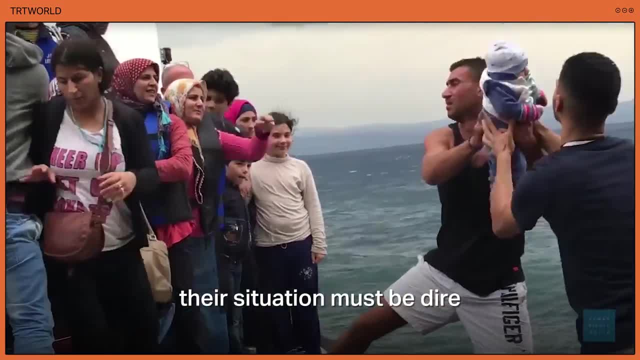 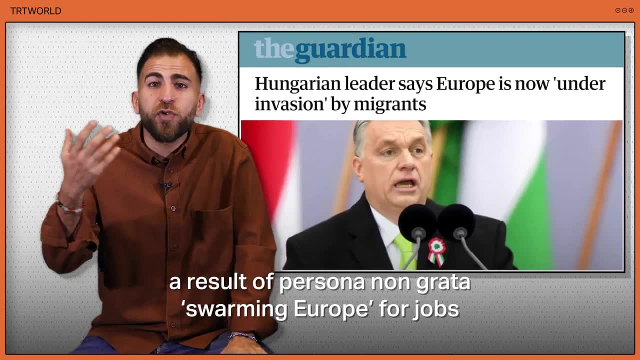 and the lives of their offspring. their situation must be dire. Forcibly displaced people are fleeing perils that the 1951 conventions drafters could not imagine. Making the crisis seem like a result of persona non grata. swarming Europe for jobs is inflammatory. 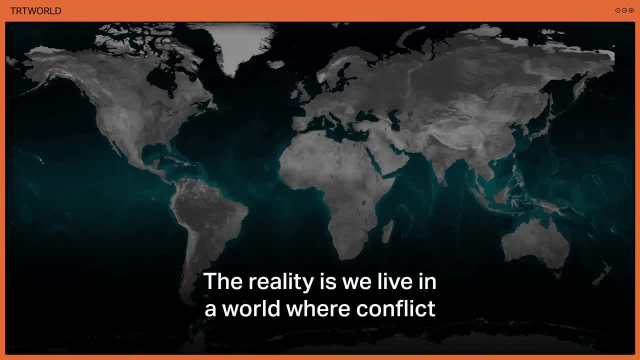 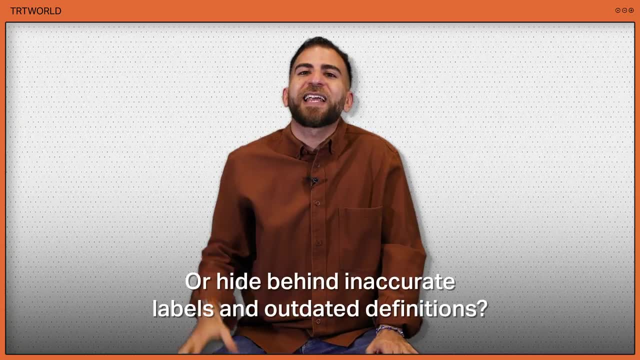 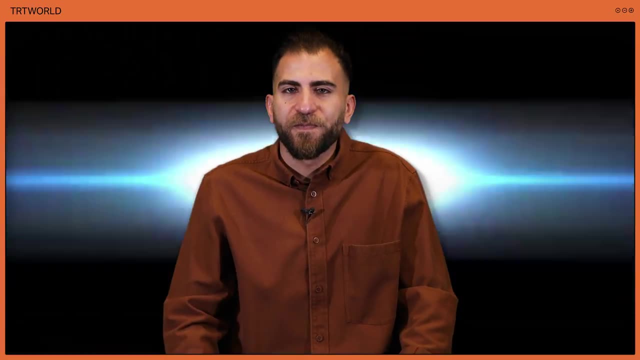 and simply not factual. The reality is we live in a world where conflict, poverty and climate change affects millions. Do we share the responsibility and help, Or hide behind inaccurate labels and outdated definitions? Thank you, guys. please make sure to subscribe and like. See you next week.